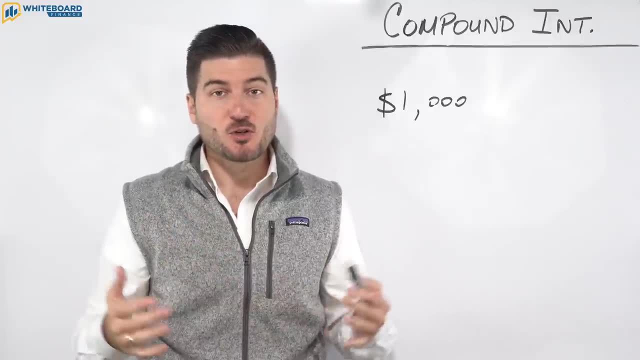 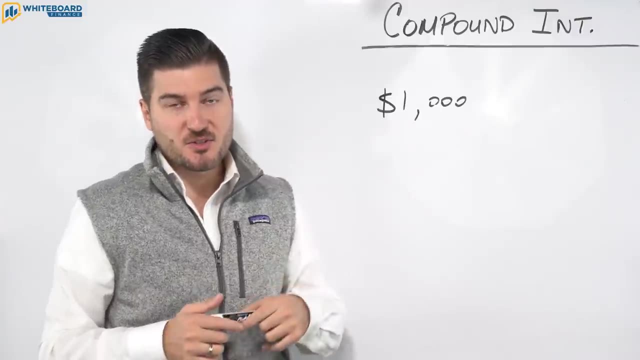 most of you watching this video right now at some point have either had a savings account or a checking account, some sort of account that earns some amount of interest. So let's say we have $1,000 in the bank. So this bank is going to pay us a 4% annual percentage yield. That means 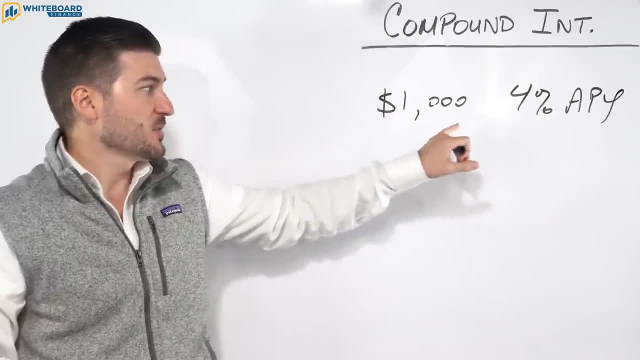 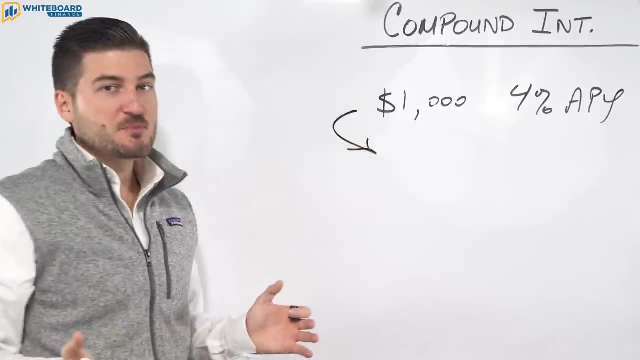 at the end of every 12 months or every year. this is going to compound at 4%. So in this quick example, at the end of 12 months, you can answer down in the comments below: how much money would you have? Well, 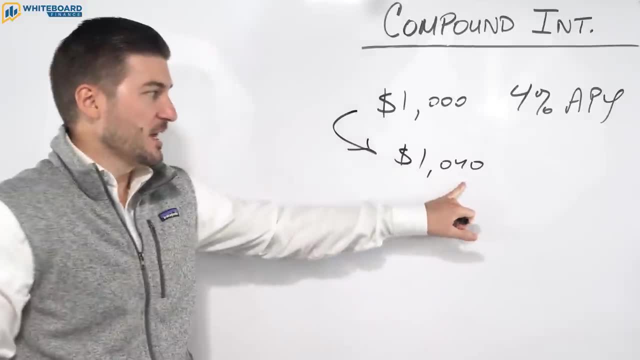 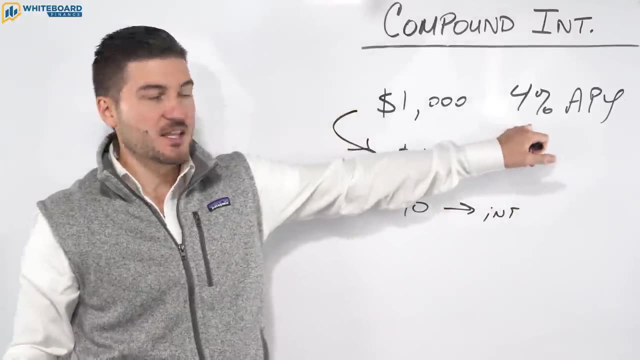 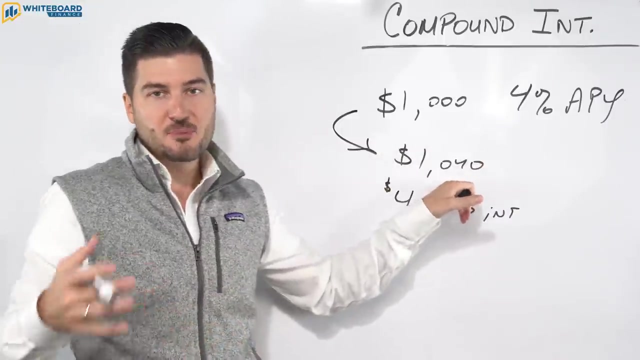 this is going to grow to $1,040.. You would have earned $40 in interest over this 12 month period, based on this annual percentage yield. Okay, So this is where it kind of gets interesting. So if I were to leave this $1,040 in the bank for another 12 months, you would obviously be earning 4%. if 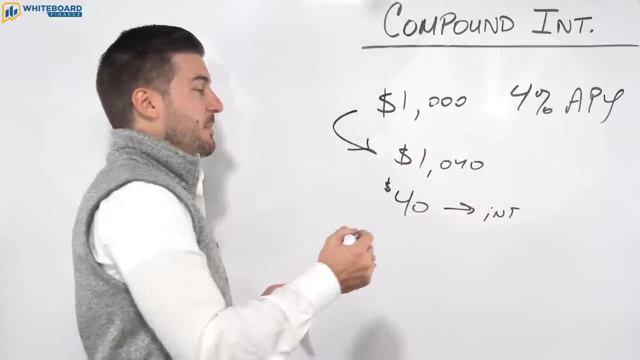 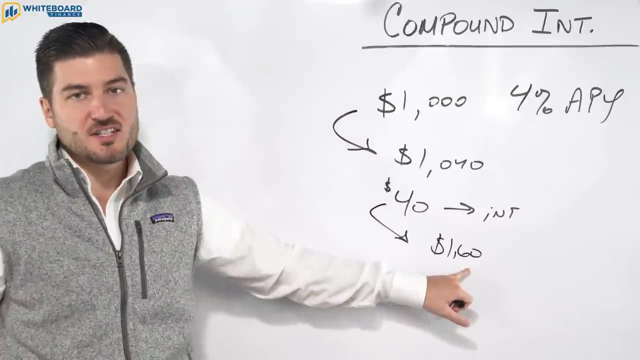 the bank doesn't change that rate. However, this is where the power of compound interest starts. This $40 over the next 12 months is going to throw off an additional $1,060.. So, yes, that's, you know a little bit more than a. 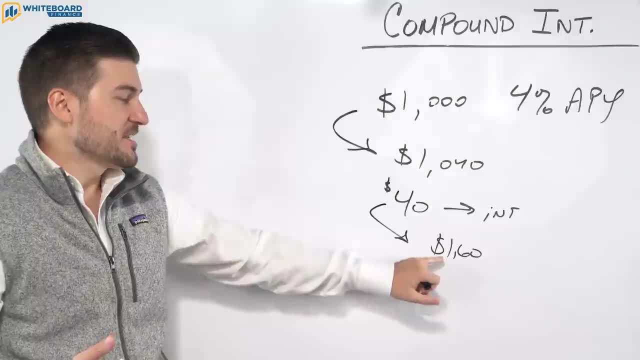 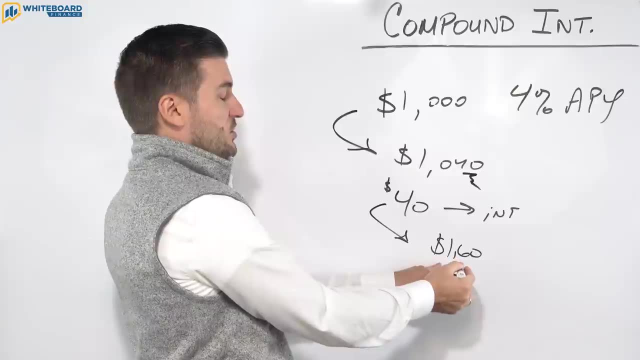 dime every month, which obviously isn't a lot, but this is basically the power of compound interest. in a nutshell. You didn't do anything to earn the 40,, which means you didn't do anything to earn the additional $1,060.. And that's where this can really start to snowball And we can show the 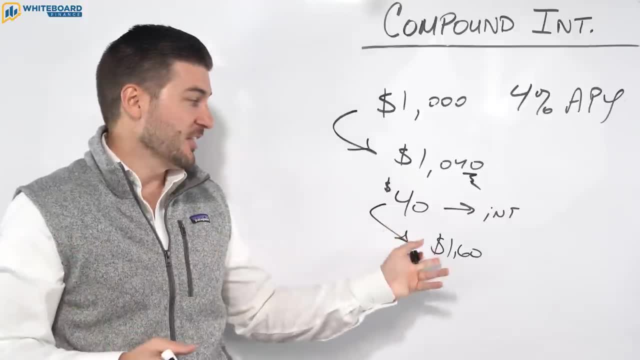 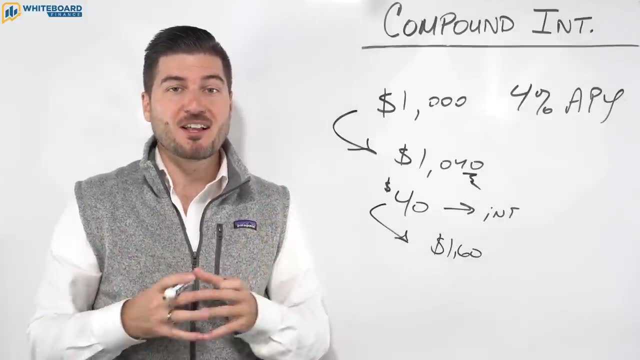 process of growing this money exponentially. And again, this $1,060 may not sound like much, but over time, with big enough numbers and compounding can deliver incredible results. Let's look into the formula and how it actually does that. Okay, So this is the formula. 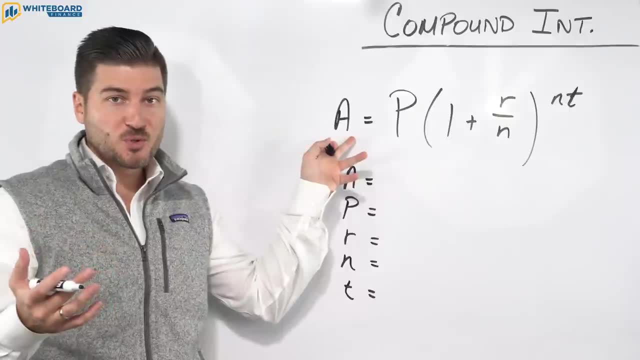 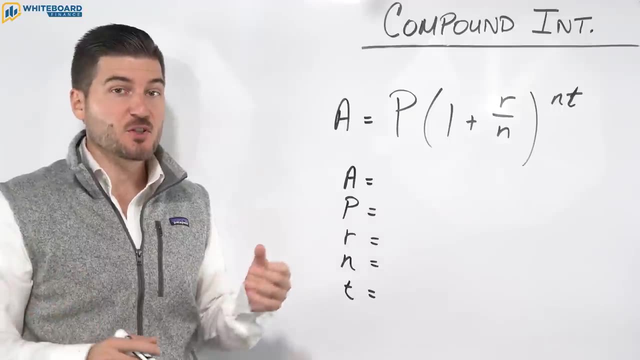 for compound interest. This is basically a. this is the total or the accrued amount. This is the principal plus interest. P is going to be the principal amount, the original thousand dollars, If we go back to the last slide's example, one plus R. R is going to be the annual nominal. 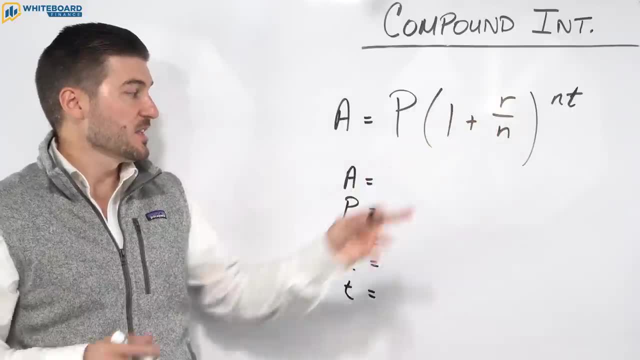 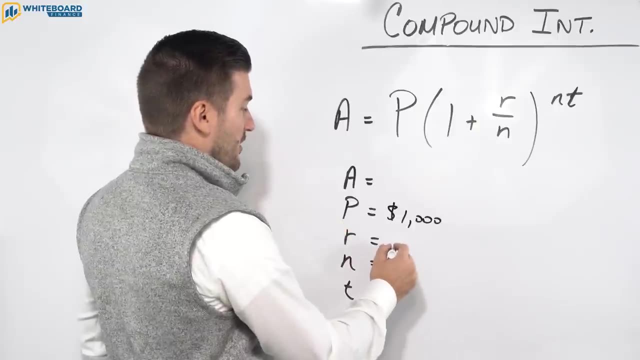 interest rate as a decimal. So in this case, if we're going to be using- actually it's probably easier if I just fill these in- So let's just say thousand dollars from our last. that's the principal. R is going to be the interest rate, So it's going to be 4%. This 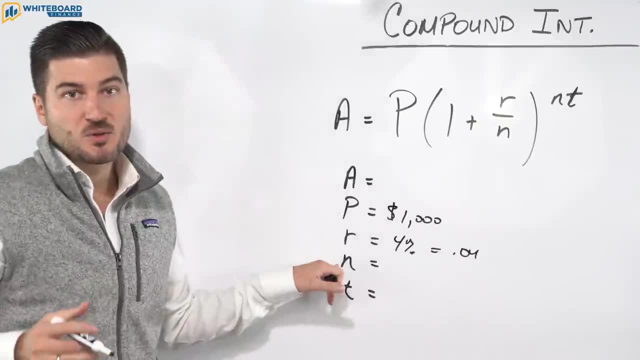 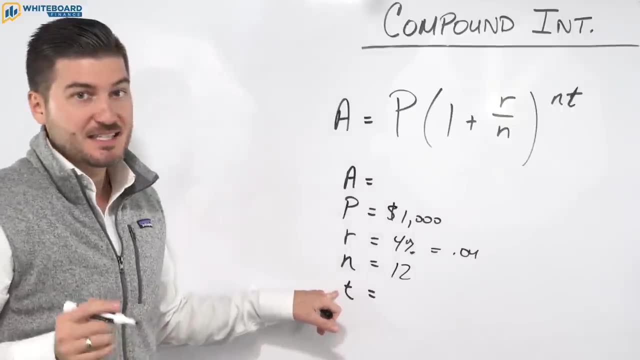 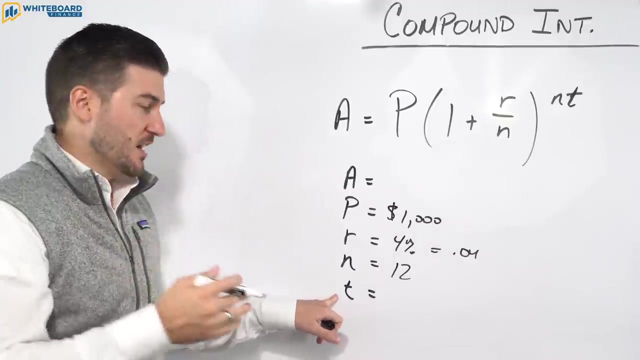 actually really means 0.04.. N is going to be the number of compounding periods per units of time, So this is 12 months. Remember, we're doing this monthly. And then T is going to be the time in decimal years. So, for example, if this was six months, we'd be using 0.5 years, Since we're 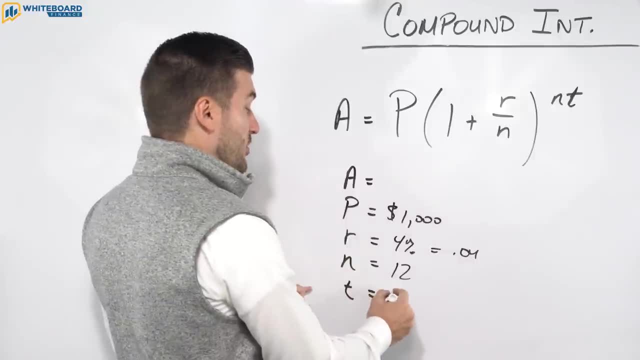 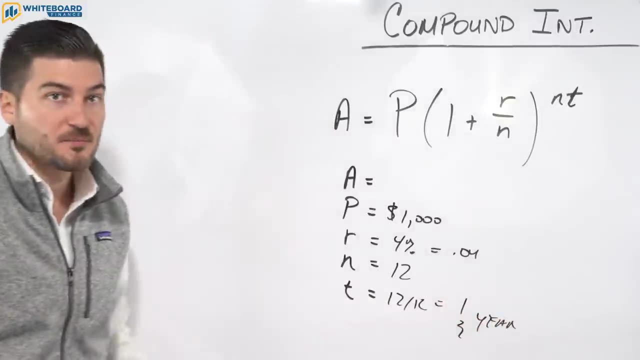 doing over the course of a year, which we use in our last example. it's going to be 12 divided by 12 equals one One year. Okay, AKA, we're using the number one right here, Okay, So, without actually doing the. 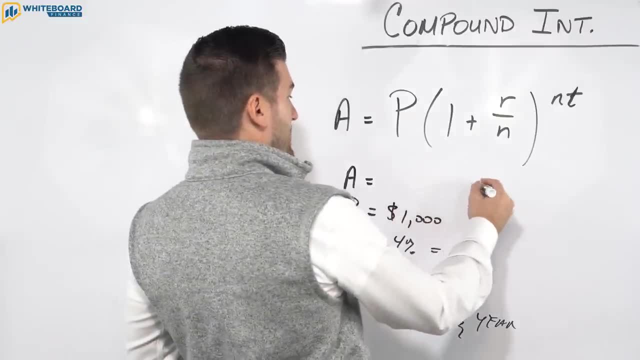 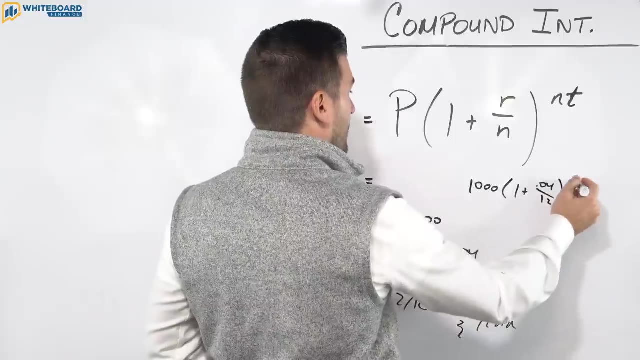 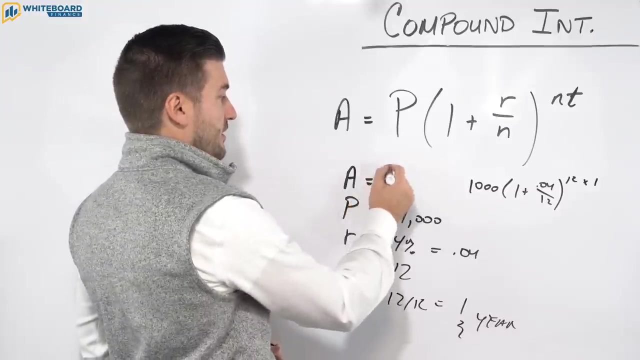 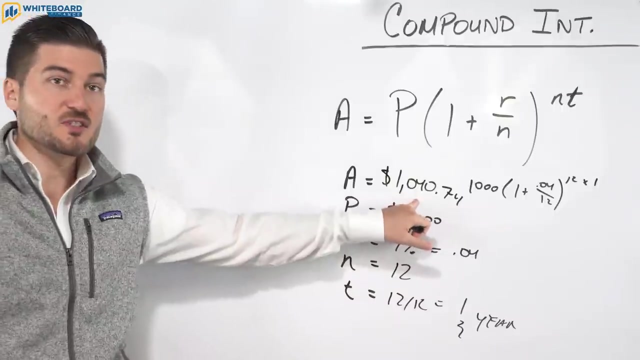 math. I'll just replace these variables So you can see P is going to be thousand one plus 0.04 divided by 12.. And then you're going to have 12 times one. So this is basically the formula to get you the answer of $1,040 and 74 cents. Okay, This is basically the $40 in interest. 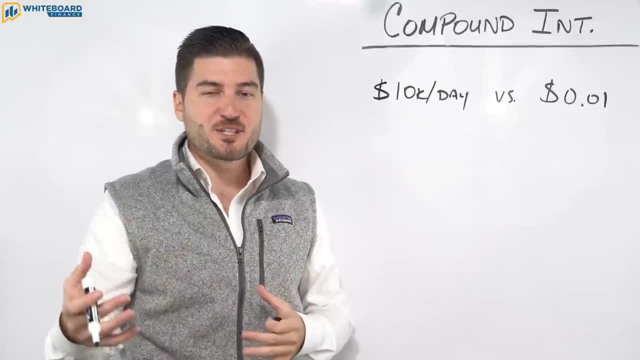 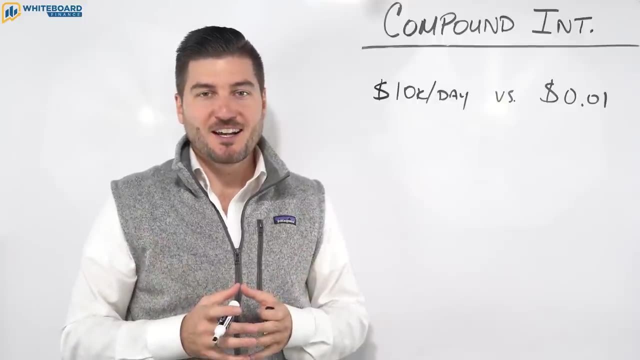 We talked about in the previous slide Makes sense. Okay, So here's the fun experiment that I was talking about in the beginning of the video. There's many different variations of this story, or this experiment, or this fable, if you will. There's one like medieval example of 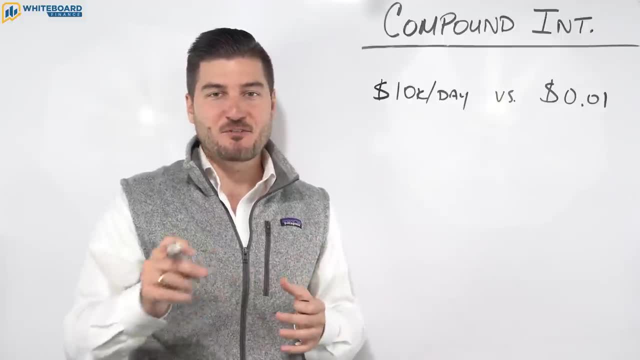 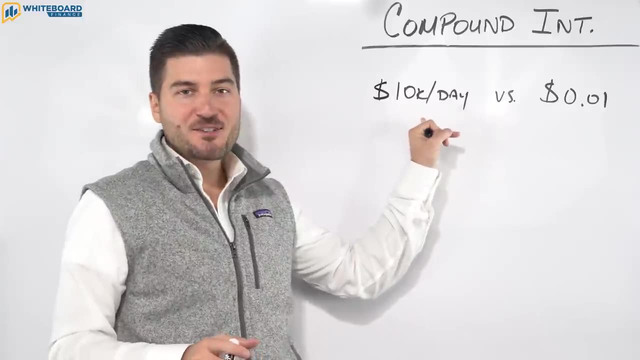 some engineer creates something He offers to double a grain of rice every square on a chess board, whatever. This one's a little bit easier to understand. So would you rather take $10,000 a day, every day for a month, or one penny that doubles each day for a month? 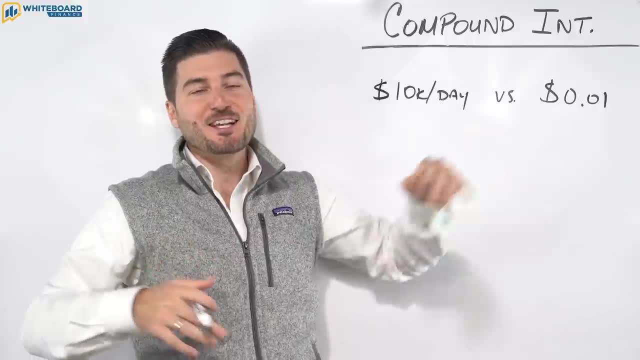 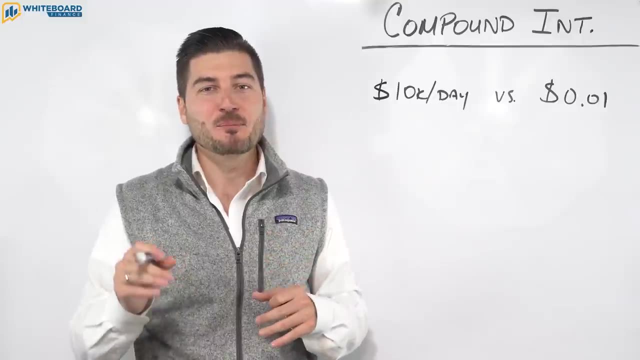 So pause the video and answer down below. Don't look this up. Obviously, you already probably know what the answer is going to be, because it's a video about compound interest. But thanks to compounding, that, penny will have doubled to this amount, And I'll show. 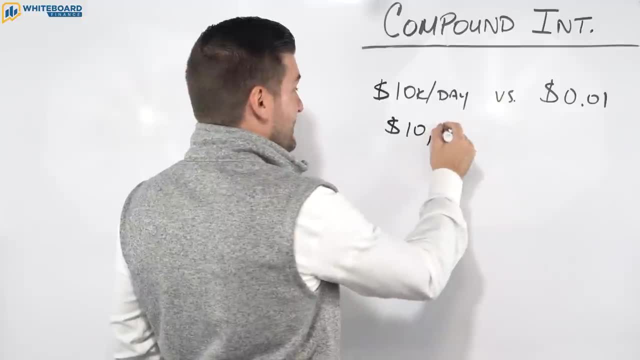 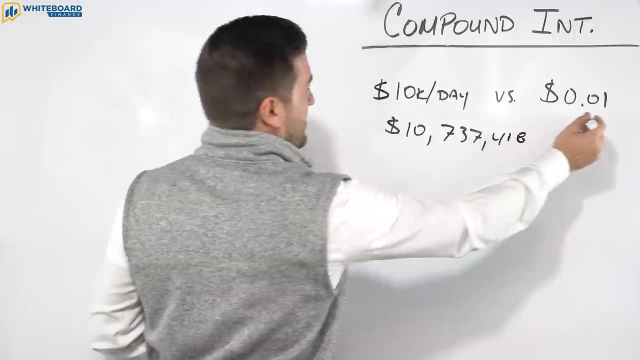 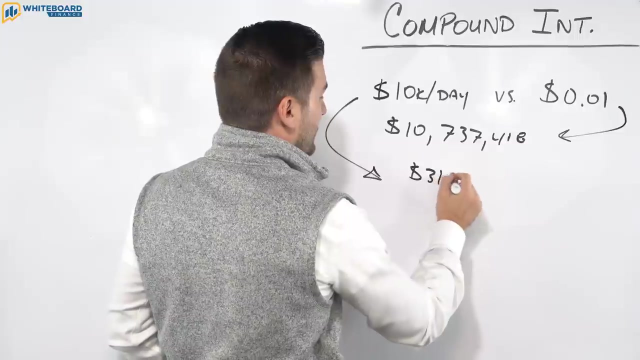 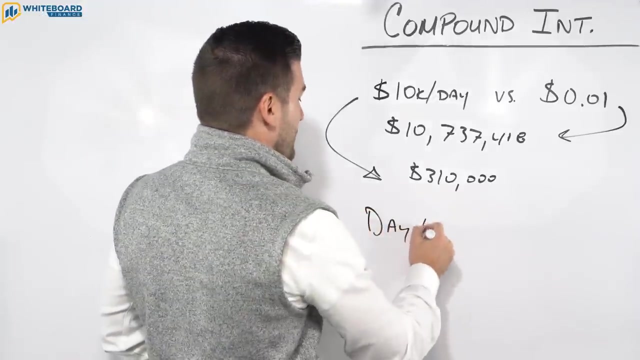 you how It's going to double to $10,737,418 versus. this is the penny doubling versus. if you were to take 10 grand a day for 31 days, you're obviously going to get $310,000.. So it's a much bigger difference. So here's something cool. So on day 15,, that penny doubling is worth $8,192.. On day 20, that penny doubling is worth $5,242.88.. So this person's laughing at you. They have grand, you have 5,200 bucks. They're like you're an idiot. Why did you do that? But on day 25,. 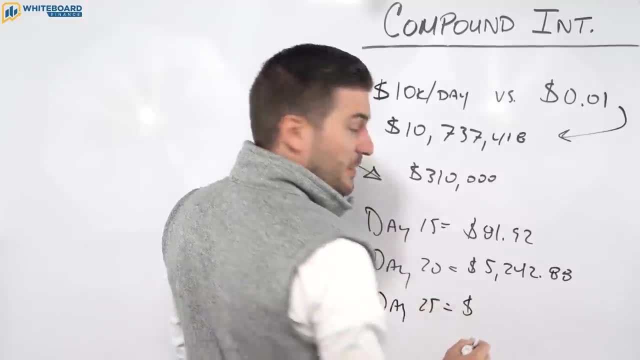 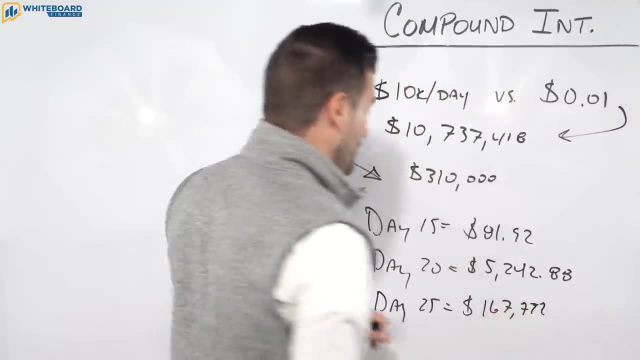 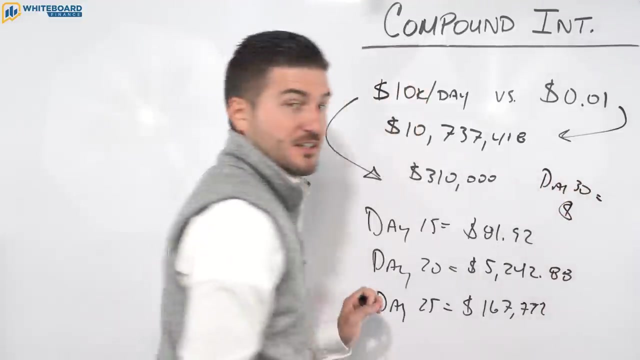 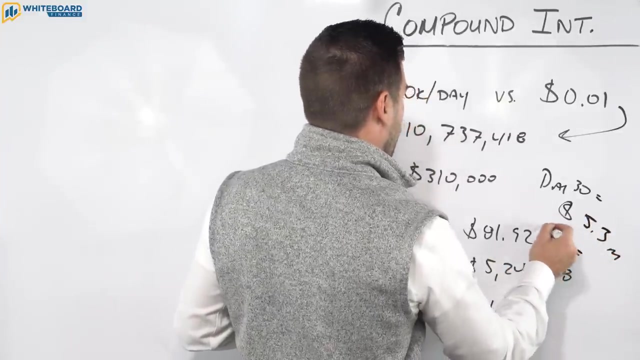 they still have more money than you They have. you have 167,772 and some change On day 30, you have 5.3 million. Day 31, you have this number right here: $10,737,418.. 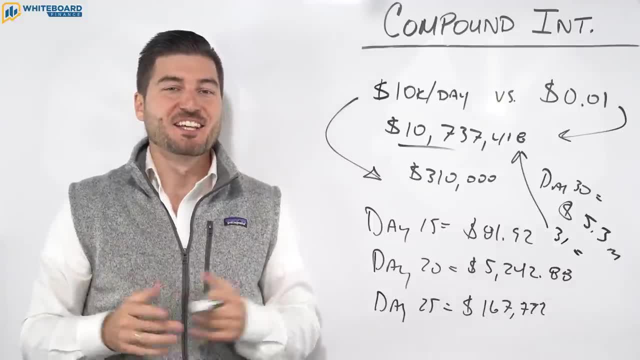 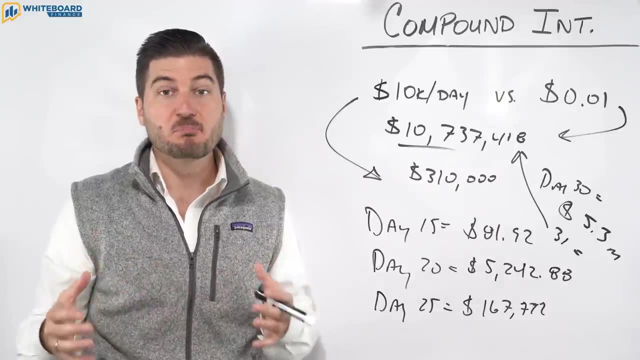 So that's the power of doubling. Obviously, you know these aren't realistic compounding terms, but it's just to show you that over such a small period of time compounding can really build. And I'll show you why in the three levers. 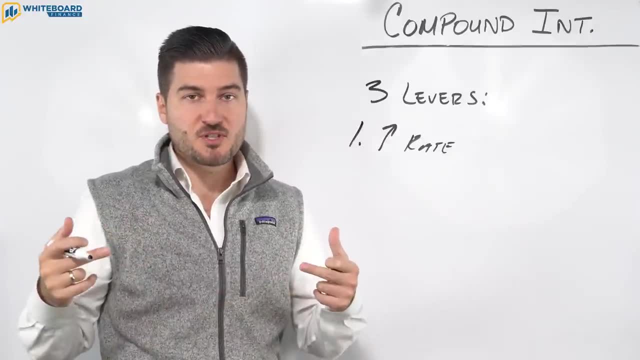 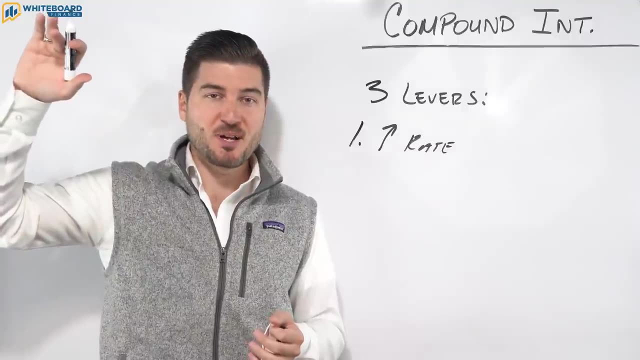 In the next slide. Okay, Here's the three levers that you can pull to obviously increase your compounding. Number one is a higher rate. Obviously, if you've been following the Fed and what they've been doing, we basically went from ZERP- zero interest rate policy. to an overnight Fed funds rate of like five and a half percent in a very small amount of time. That's why high yield savings accounts rates are going up like crazy. So here's an example. Let's just say for big numbers, you have a million dollars at 4%. This is obviously going to throw. off $40,000 in interest after a 12 month Period. If you go to a higher yield savings account- or you can somehow increase this yield to 5%, this is no brainer- turns into 50 grand a year. Okay, So you just made an additional $10,000. 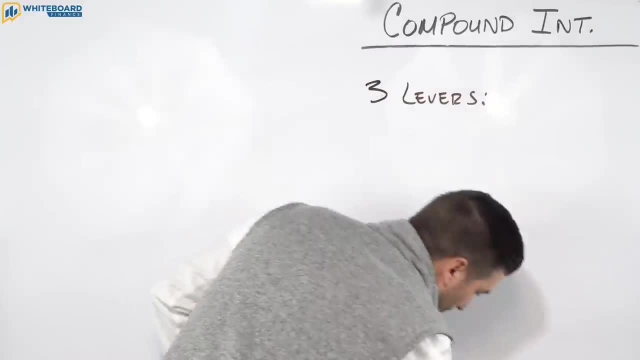 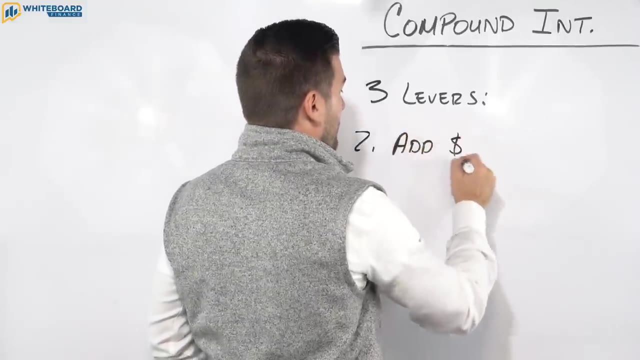 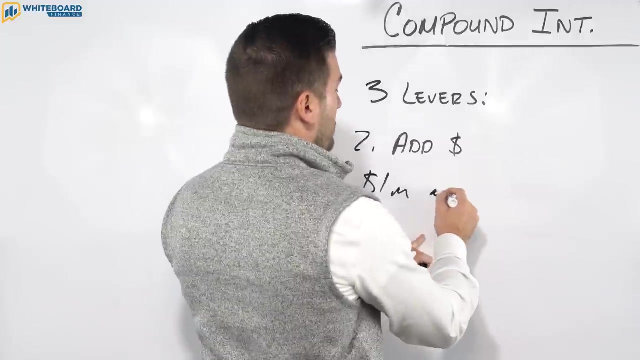 Okay. So number two: we're going to add more money along the way, So add money. So if we take that example of a million dollars and we actually start to throw in, we'll, we'll keep this at 4% and we start to throw in 5k a month. I know this isn't realistic for most. 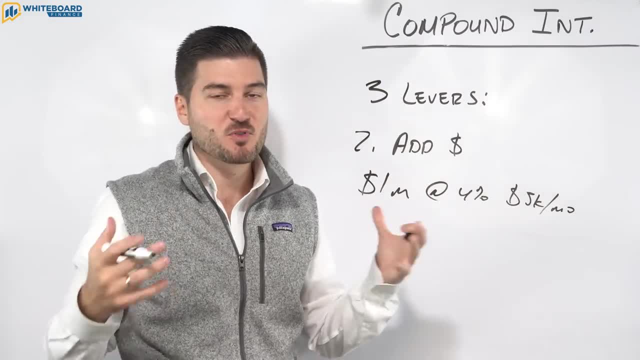 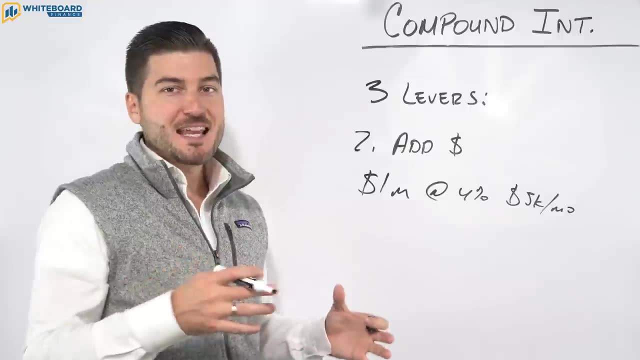 people watching this video. I'm just doing this, So the number's bigger and it makes more sense to prove a point. So, on top of the 40,000 that you're already going to make if you had an additional $5,000 a month, every month, that same million is now going to be worth 1.1 million. 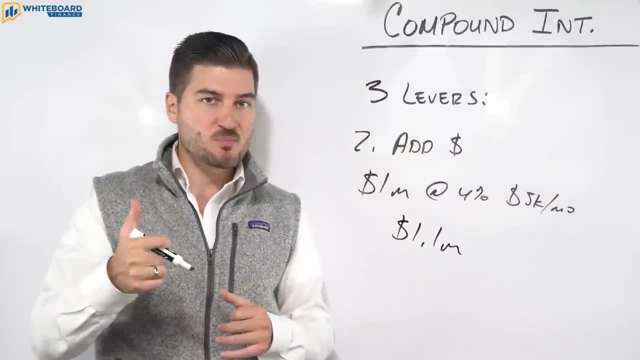 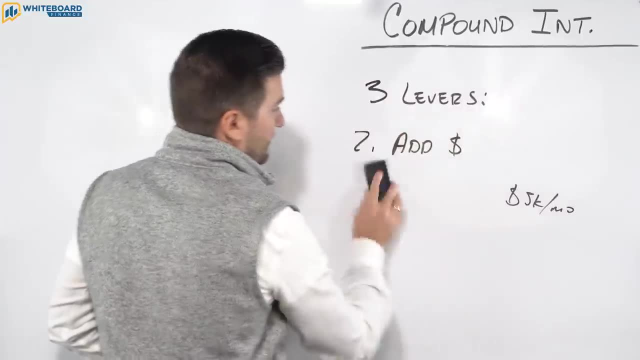 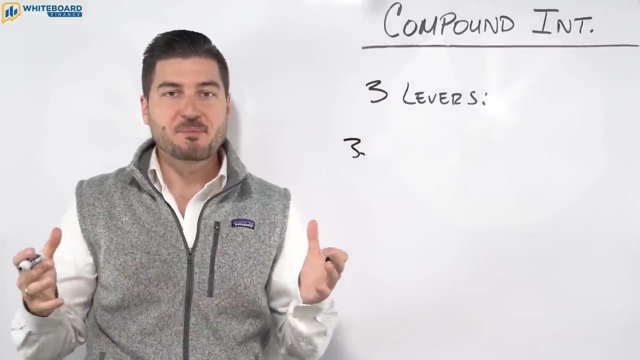 actually a little bit more. I just don't want to write out the whole number between the extra interest payments and also the $60,000 a year contribution. Okay, So this is obviously. another option is to add more money. Number three is patience. So if you give your money time, 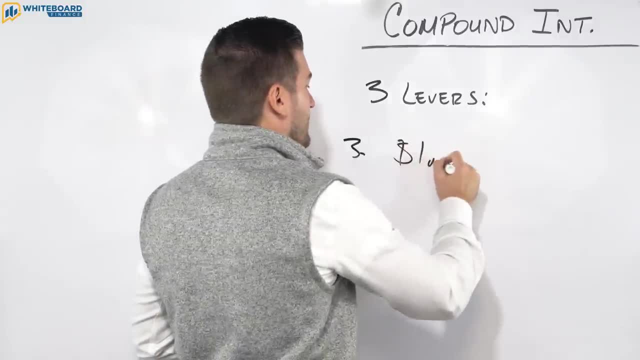 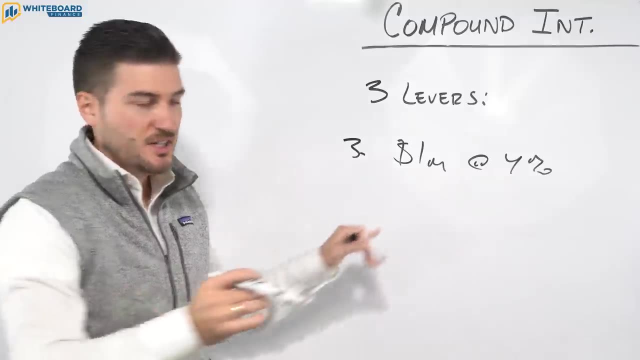 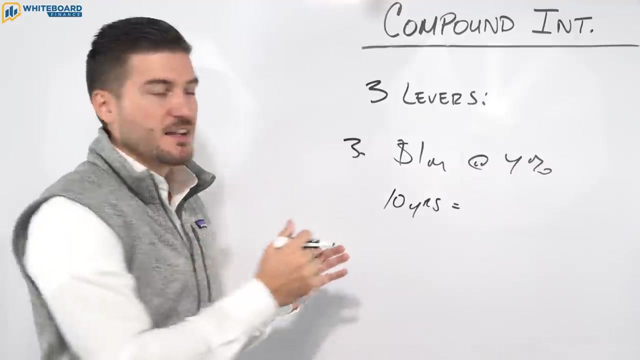 to compound and grow that same million dollars. let's just say at 4%. if you, if you didn't touch it, if you just threw in this million bucks and didn't touch it, this is going to become over 10 years And you can plug this all into the formula we just learned about in the last slide. This is: 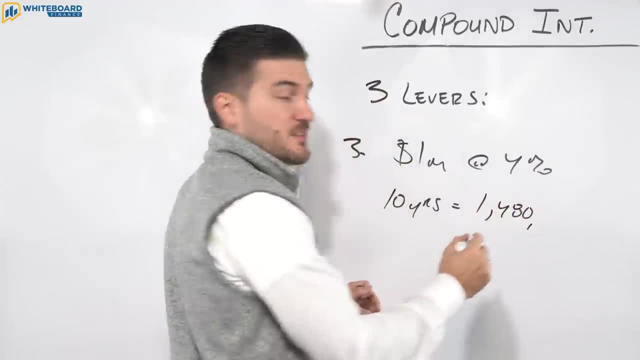 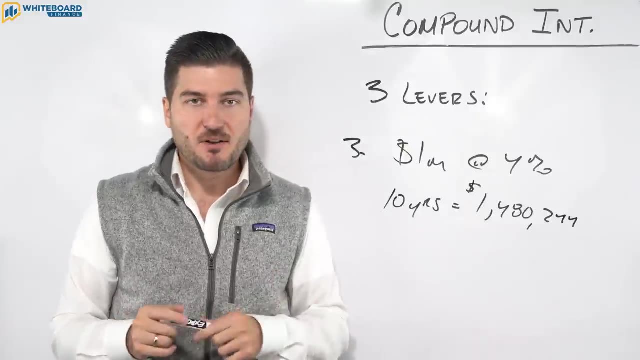 going to become 1,480,000. $244 by doing nothing in 10 years. Now we'll talk about some of this stuff- Why compounding may not be as powerful as it used to be- And we'll get into that right now. Okay, So let's get into. 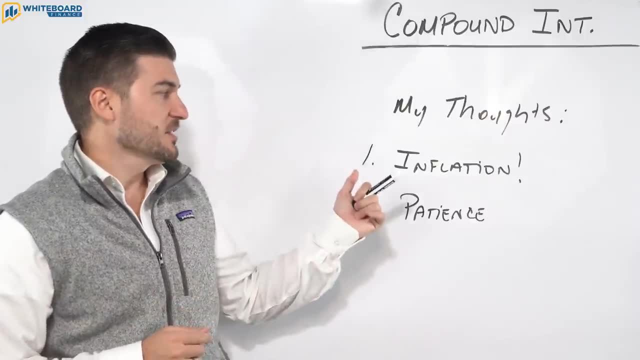 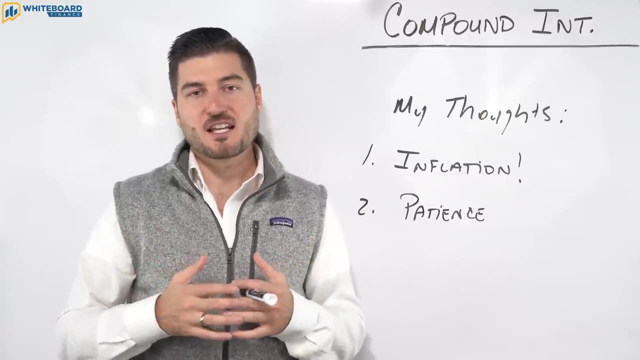 my finishing thoughts for this video or my final thoughts. So basically, there's two things I want to touch on. Obviously, the elephant in the room is inflation. So it doesn't matter if you're earning four or 5% in your high yield savings account if the cost of groceries are up 20, 30%, right. 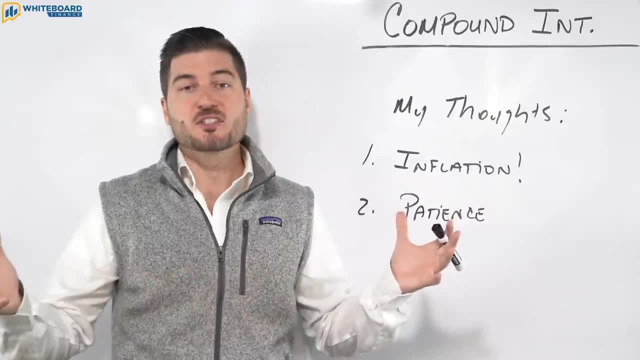 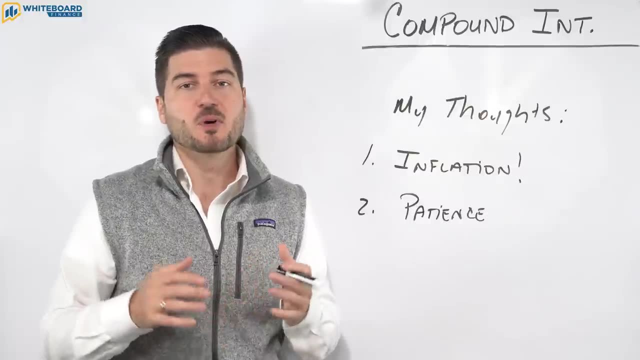 Or the cost of going out to eat is 20, 30%, or you know your CPI is 20, 30%. So that's obviously an exaggeration- Not in some cases. some groceries actually are up that much. but what I'm trying to say is it doesn't matter if you're compounding interest, if CPI or the 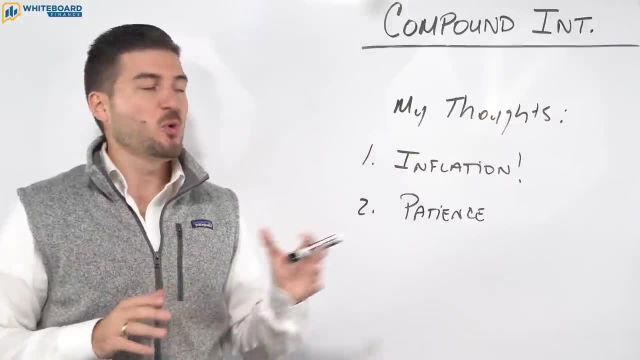 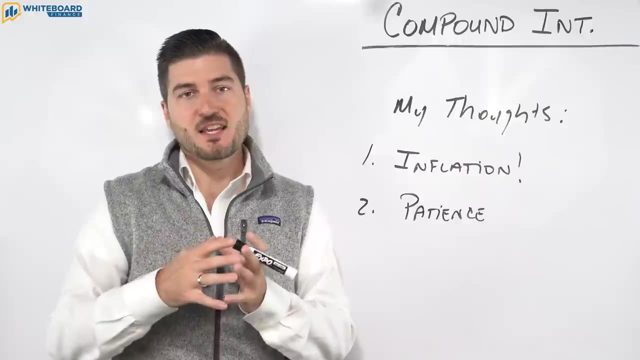 cost of other goods are compounding as well, right? So my point is is that if inflation is 5% and you're earning 4%, you need to figure out a way to make a difference on that 1%, right? Which kind of brings me to my second point, which is patience. So don't pull your money out. 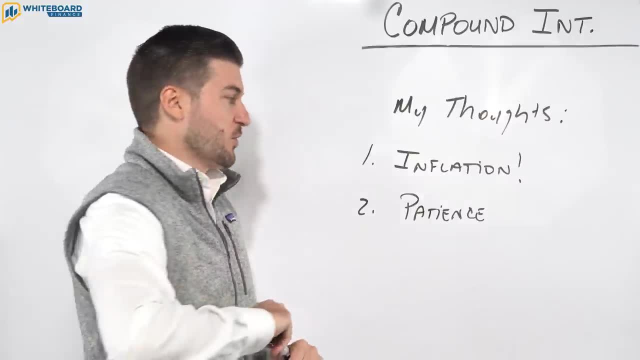 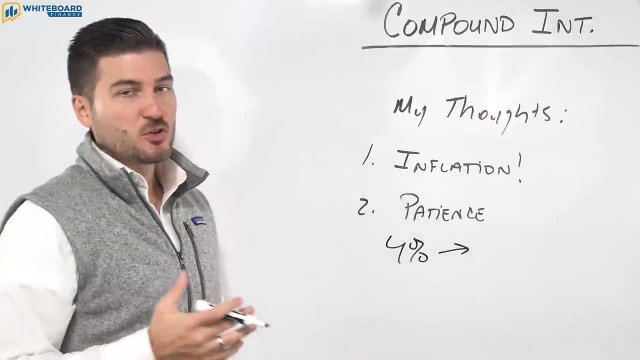 unless you have a better opportunity to invest. So if, going back to that example of 4% that we used throughout this entire video, your friend comes to you and says he has some- you know- miracle tree in his backyard and it throws off a guaranteed, you know, 7%, you know, obviously you need to put your money where it's. 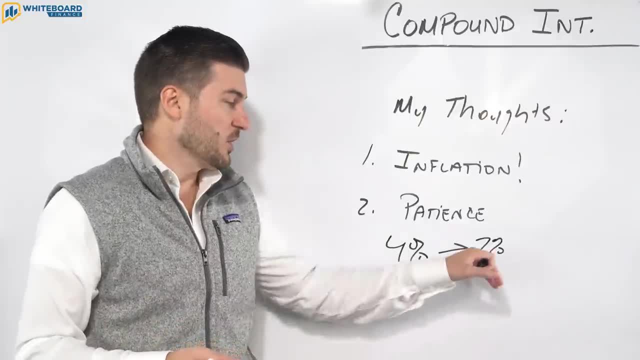 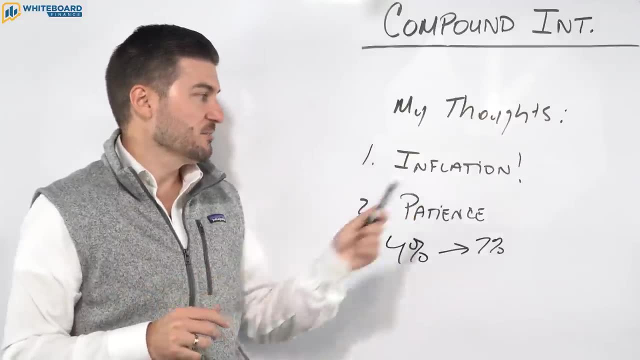 best treated and get the highest rate of return. These are 100% passive opportunities. Why would you settle for 4% when you can make 7%? So it's kind of like the inflation point, just in reverse, if you will. However, these both 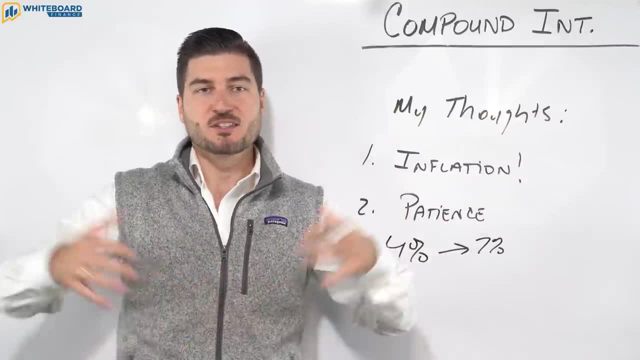 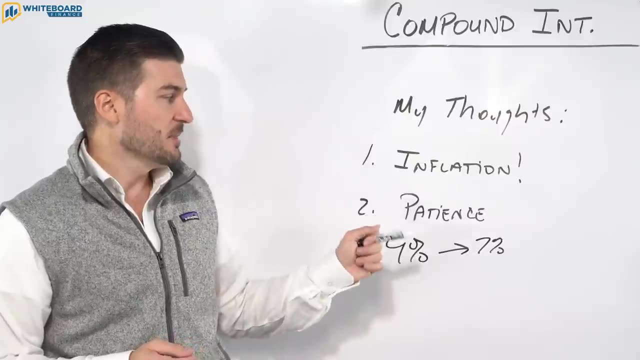 Trump, leaving your money under a mattress, in a vault, in the drywall of your house, because then you're just getting destroyed by inflation. There goes your purchasing power. So, compound interest: you're going to benefit by defeating inflation, maintaining your purchasing power and also being patient by putting your money in the right things. 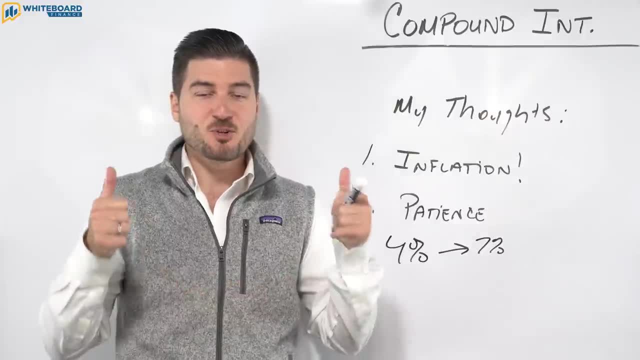 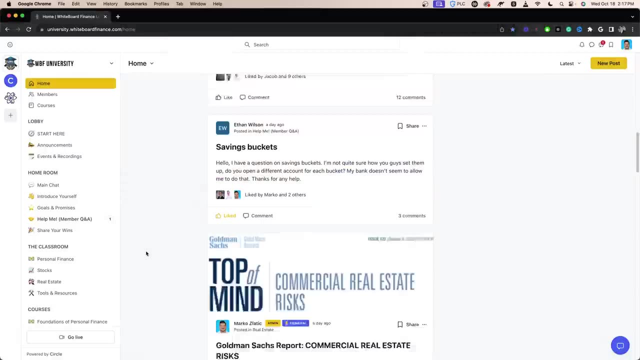 Thank you so much for watching. Hopefully you got value out of this video. If so, please share it with a friend, give it a thumbs up, like and subscribe, if you haven't already, And also check out Whiteboard Finance University. I'm giving a 20% off coupon code.